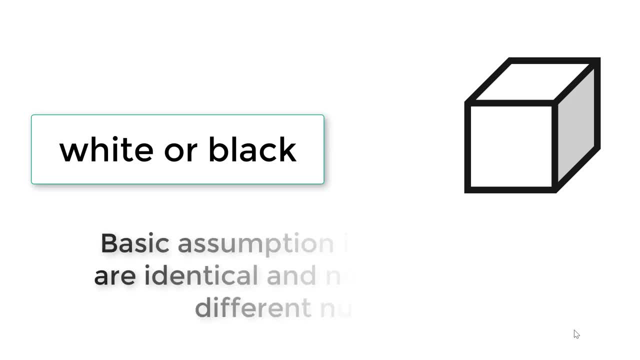 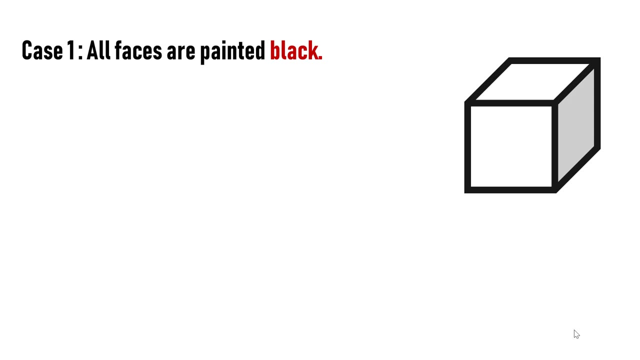 Hence there are many cases possible. Basic assumption is that all faces are identical and not identified by different numbers. Let's consider different cases and analyze the problem. In case 1, let's assume all the faces are painted black. In this case, total possibilities is only one, because you can paint all faces with black only in one way. 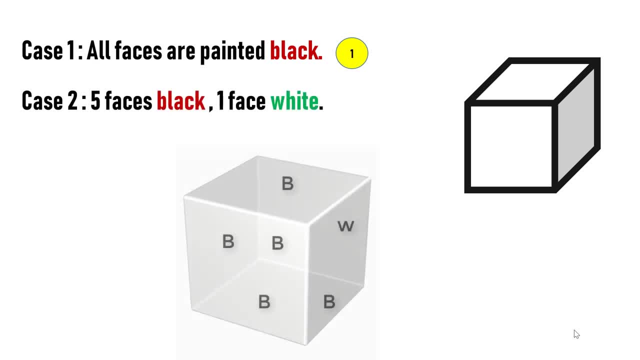 In case 2, let's assume 5 faces are painted black and one face is painted white. In this case there is only one possibility, Since cube is symmetrical figure on all its faces. that is why 6 cases will reduce to 1.. 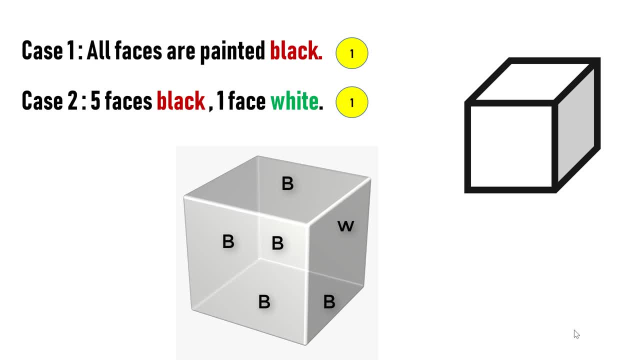 That is why there is only one possibility. That is, even if you paint white on all faces at different instances, it looks same. In case 3, let's assume 4 faces are painted black and 2 faces is painted white. 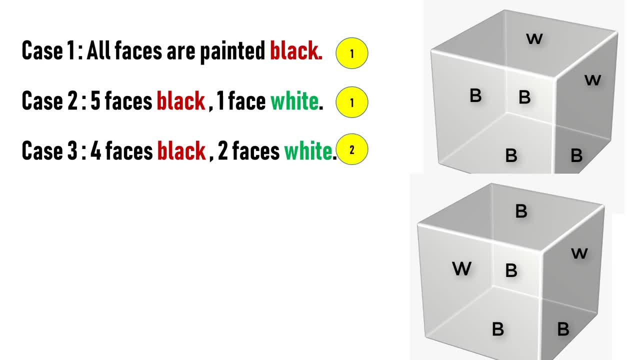 In this case there are two possibilities: The first when the two white faces are on opposite faces and second, when the two white faces are on adjacent faces. If you paint two faces with white at any number of instances, there will be only two possibilities in the way it looks. 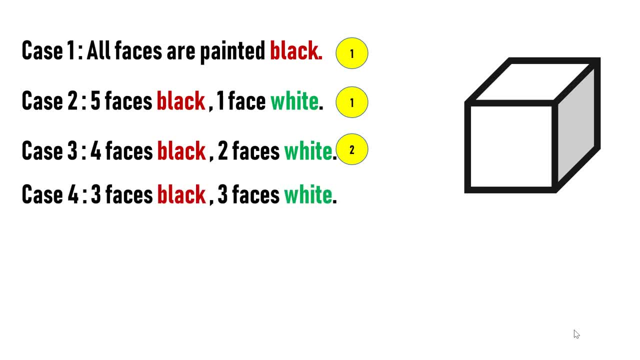 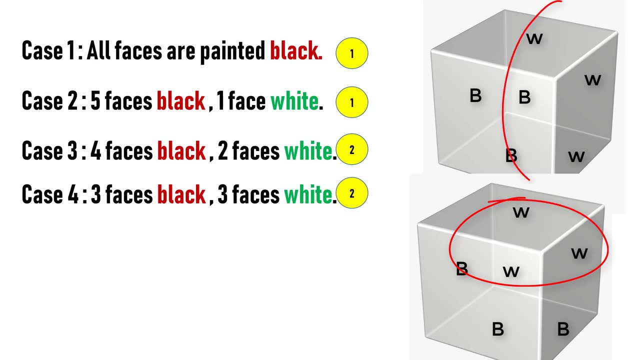 So in case 4, let's assume three faces are painted black and three faces is painted white. In this case also, there are two possibilities: The one way where three white sides have same corner, and other way where opposite sides are white and one center side is white. 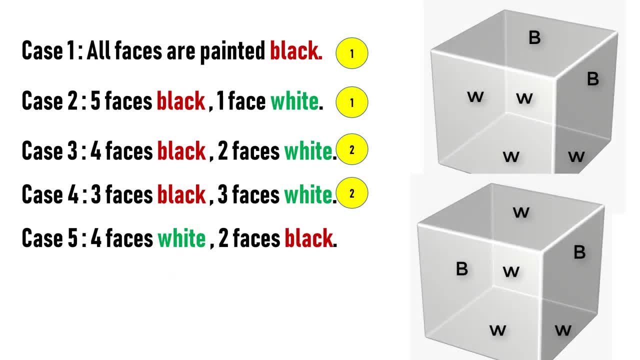 In case 5, let's assume two faces are painted black, painted black and four faces is painted white. This is similar to case 3.. So in this case there are two possibilities: The first, when the two black faces are on opposite faces, and second. 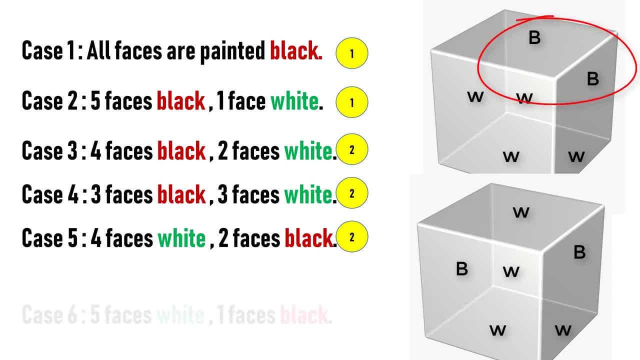 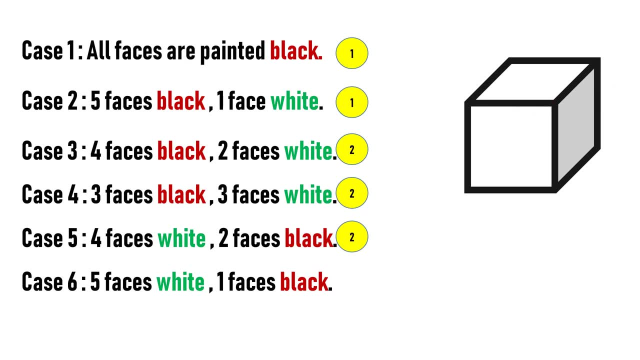 when the two black faces are on adjacent faces. In case 6, let's assume one face is painted black and five faces are painted white. This is similar to case 2.. There is only one possibility, Since cube is symmetrical figure on all its faces. that's why six cases will reduce to one. So in case 7,